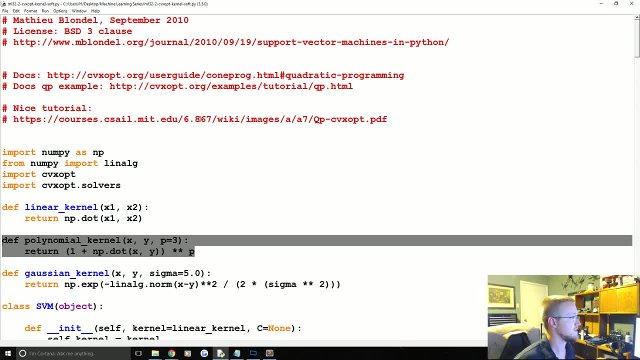 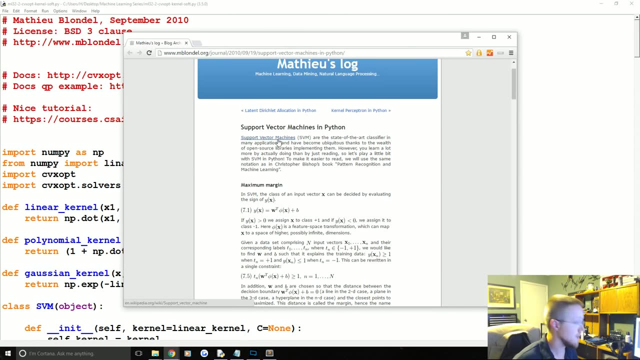 makes and also some pretty nice visualization. So this is not my code. I grabbed this from Matthew Blondell's github. Also, there's a nice blog post on this, exact how he kind of came up with this. Also, I believe, a link- possibly no, but also at least a reference to Christopher Bishop's. 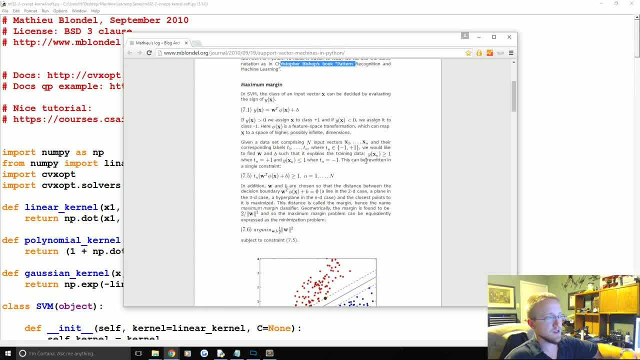 pattern recognition machine learning book and this kind of models, some information from that book as well, So you can check that out if you want to learn more about working specifically with CVXOpt. I will just say, though CVXOpt it's, it's useful in this case, just purely. 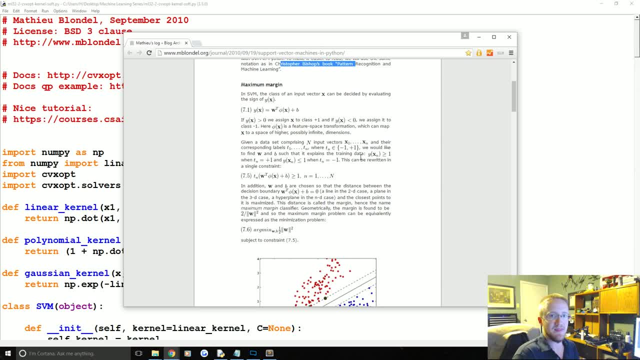 so you can see directly the impact of a kernel and where it's actually being injected and chain and modifying the initial formal support vector machine. But beyond that, honestly, CVXOpt is not something you're probably ever going to use and even like for a support vector machine if you 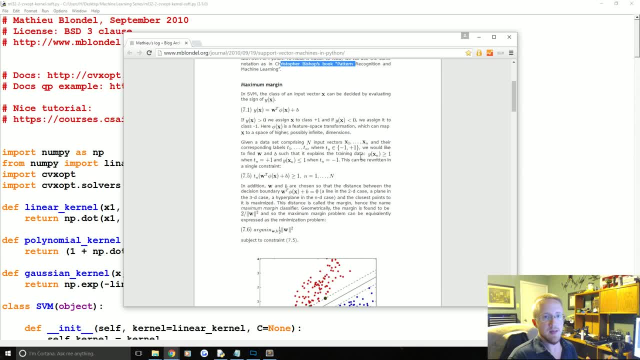 wanted to write your own, you would almost certainly be using lib svm, So just keep that in mind. but mostly this is for educational purposes, for looking at the kernels, how they affect your effect, and also visualizing non-linear and also visualizing the soft margin. You can do that in. 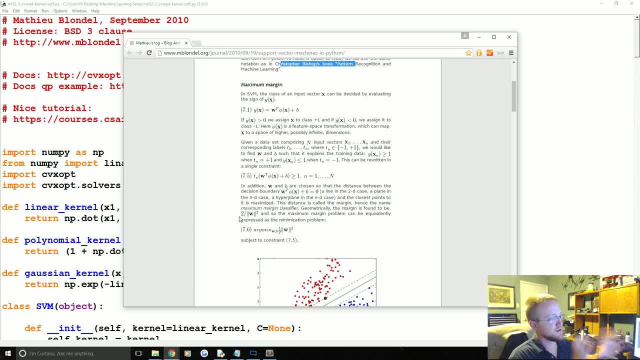 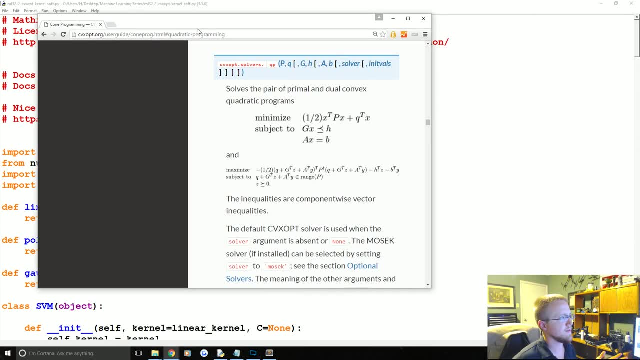 scikit-learn too, no problem, but you also. it's just a little harder to actually see the kernels impact. Anyway, head there, you can check that out. Also, there is this. I'm pretty sure we've already linked to it before, but anyway, see, this is the actual quadratic programming solver that we're. 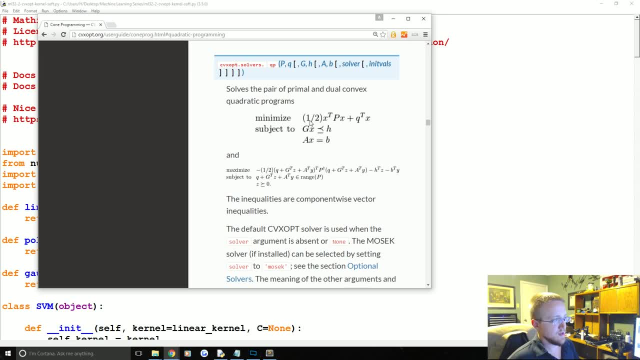 going to use It. just does this really bland equation basically, where you just you stuff in whatever values for these variables and you can see that it's actually a really bland equation. So it's just minimizing one half: x to the power of t p times x plus q to the power of t times x. 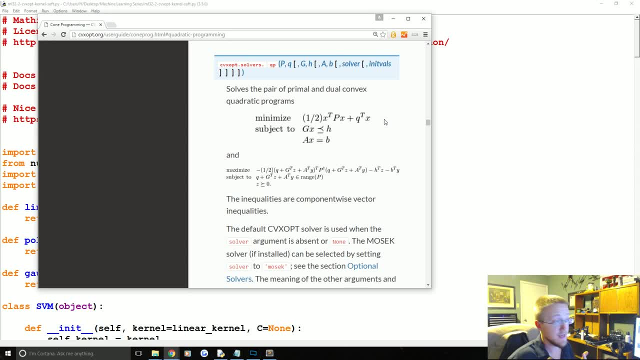 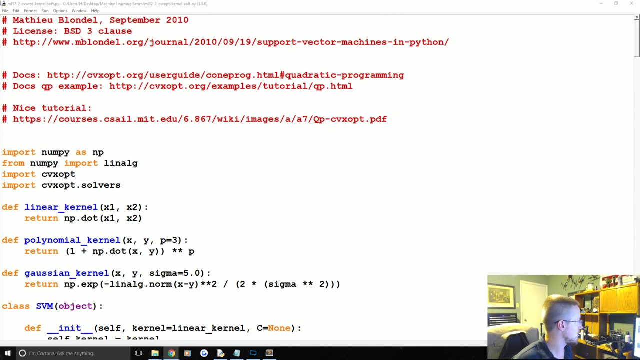 subject to. so these are the constraints. g of x is less than or equal to whatever you want h to be, and then a times x equals b, Simple enough. So, anyways, that's the solver that it runs. again links in, hopefully, the description, but also in the sample code. So, or the text-based tutorial. 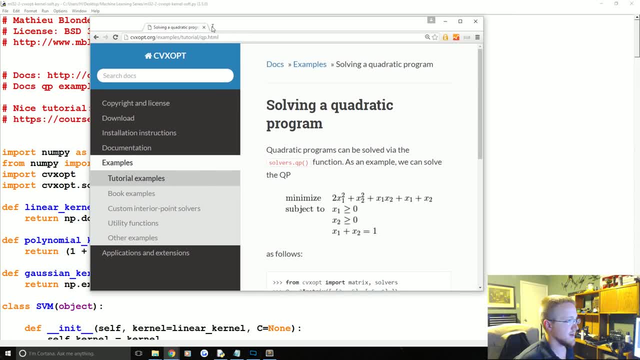 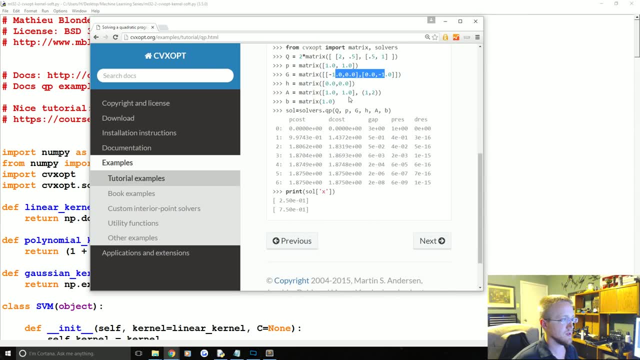 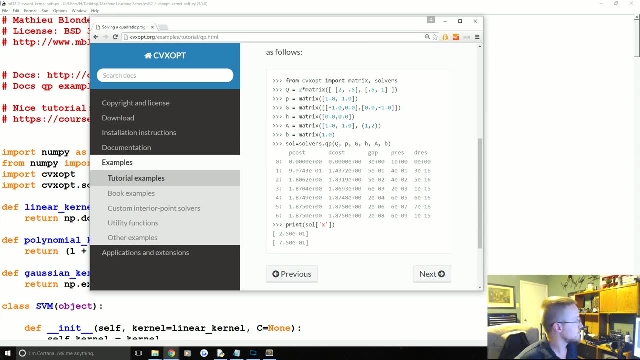 Also you can check out. there's this from actualcvxoptorg, just solving a simple quadratic programming problem. So you can kind of check that out with a really simple example of how you might solve. you know, push everything through, but you can just look at that right now and kind of get the gist. Also there's an even larger tutorial. 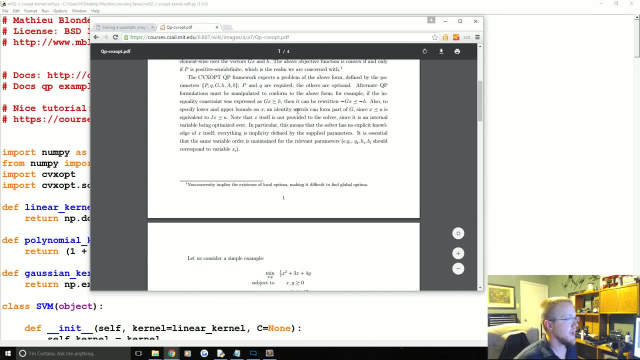 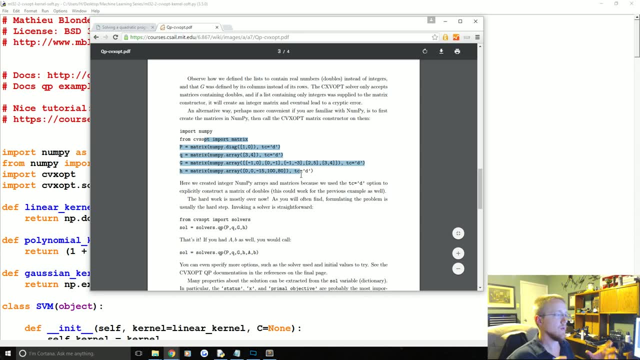 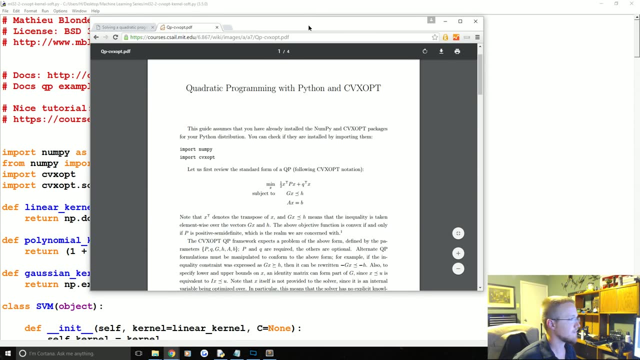 right here. I'll link to this one as well, from MIT, and it's just four pages, but it has a. it's a little bit more in-depth as far as how the solver actually works. So if you're interested in learning that, check out this, this little tutorial. here Again, links in the description and on the. 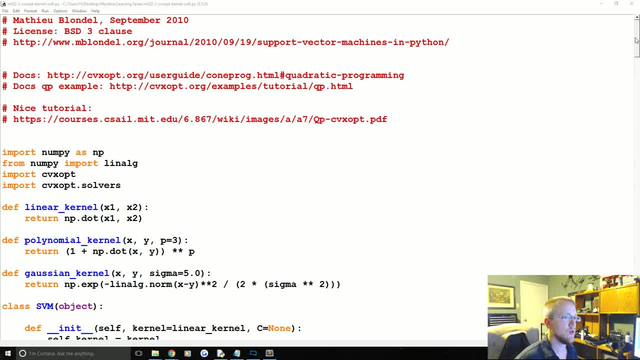 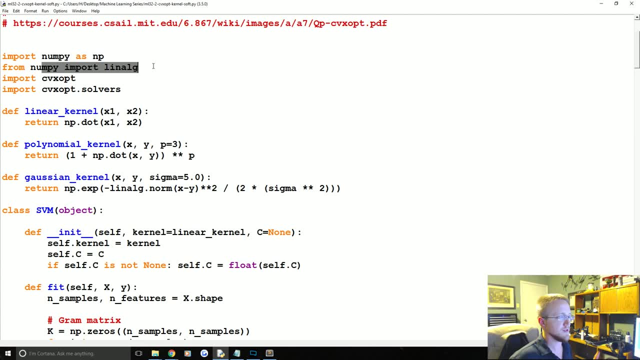 text-based version. So we're going to run through this code really quickly. but you can see, here we've got import numpy as np and then we're bringing in linalge, just specifically. we just use numpy dot linalge. but he wanted to have that extra savings of np dot. All right, import cvxopt. 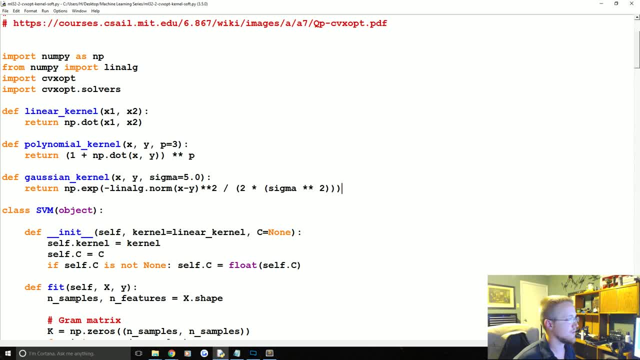 and then the solver. we kind of already talked about that. Then here's your kernels. really simple, Really talk about the Gaussian kernel, but you can look that up and you can also just see its np exponential minus linalge, norm x minus y to the power two divided by two times sigma, whatever it. 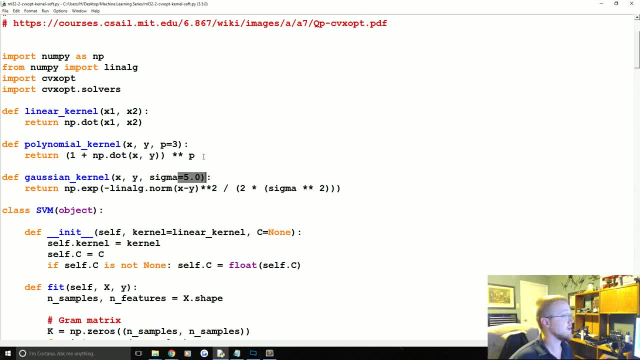 is in this case five. oh to the power. two, All right, but anyway the polynomial kernel should look really familiar- one plus the dot product of x and y- We use rather than y, x prime, but doesn't make a big difference. and this is just to the power of p, where the default is three. but you 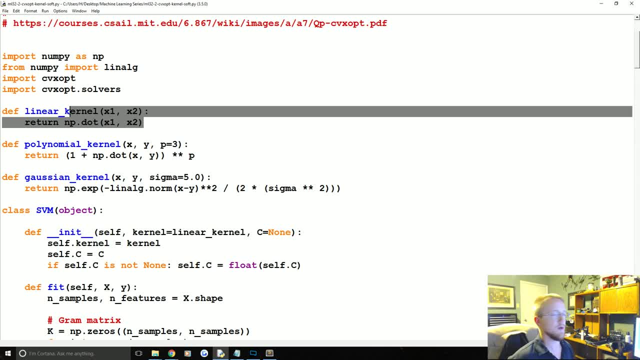 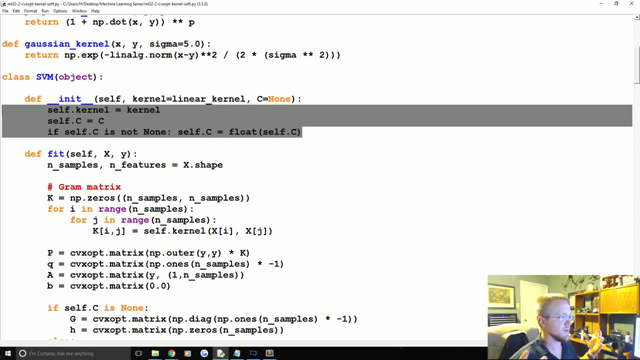 can put whatever you want. Linear kernel, That's just the original formal kernel. It's got these svm objects, no problem. the initialization method just simply sets the kernel set c defaults to none and in this case, if c is none, this is a hard margin support vector machine. So if you want to be, if you want it to be soft margin, you just 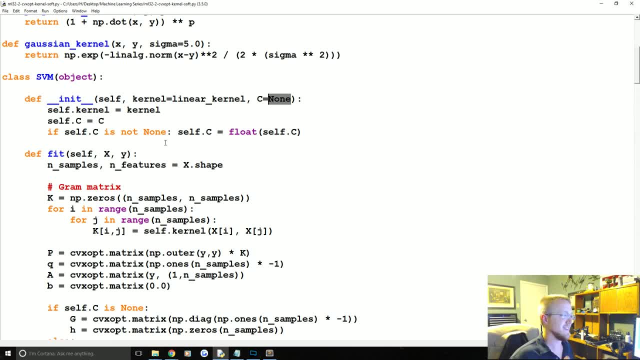 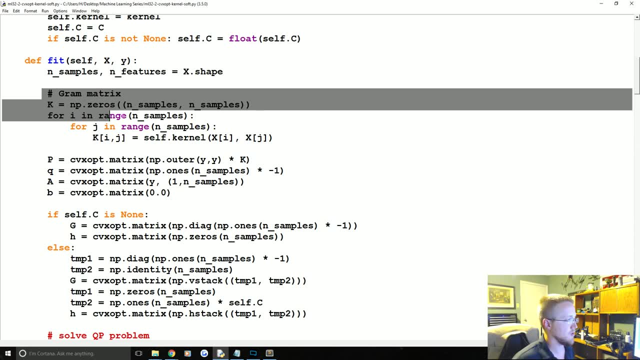 set c to something right, whatever you want that penalty parameter to be, parameter to be Coming up. next we're going to look at a little bit more about the quadratic programming solver. Basically, he's just creating all the values for that quadratic programming solver. again, this would 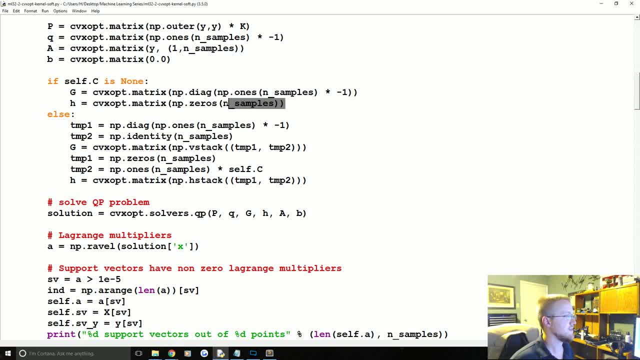 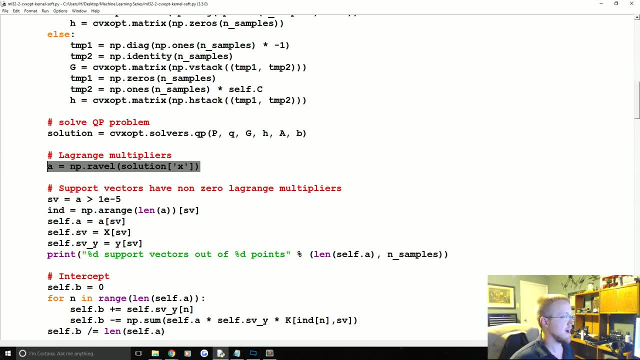 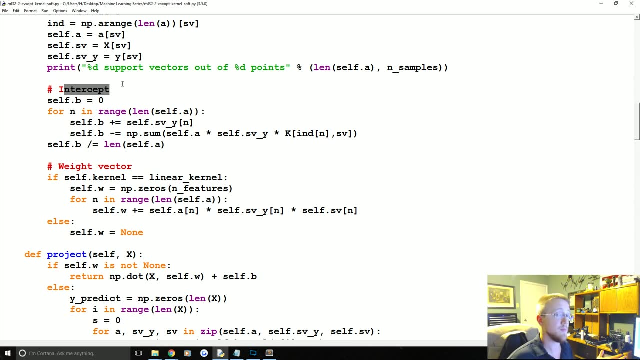 be. you know, if, if it is a soft margin, then great, and if not, then we're going to use these other values- Solves the problem, gets your solution, gets your alphas here. finds your support vectors, all that tells you how many you've got. finds the intercept which is your b, your bias, whatever you. 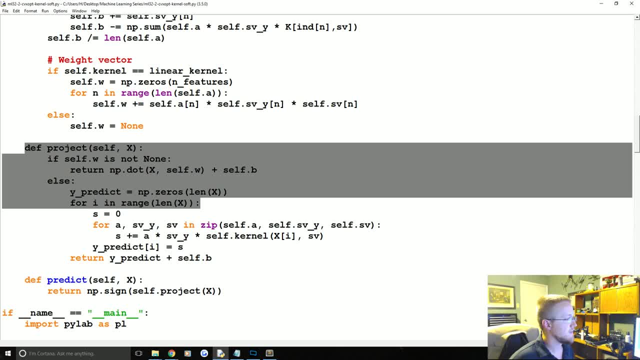 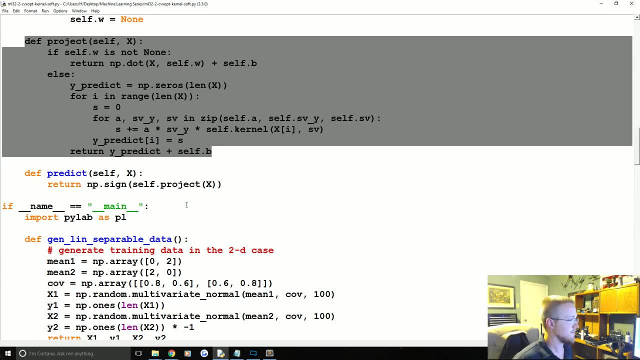 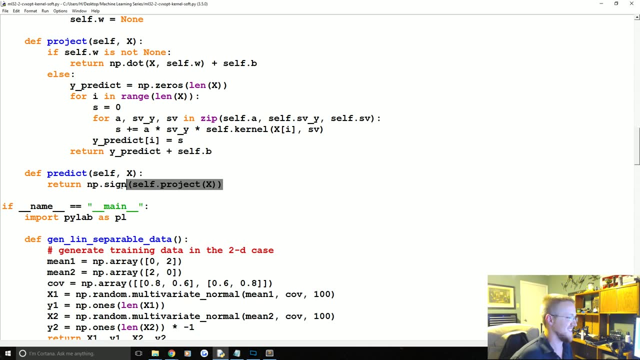 want to call it, finds w great projection. This really is only useful for, as far as I know, where is getting your prediction. And sure enough, that's basically all the prediction method does. is actually just does projection and just returns the sign of that projection. so nothing major there. 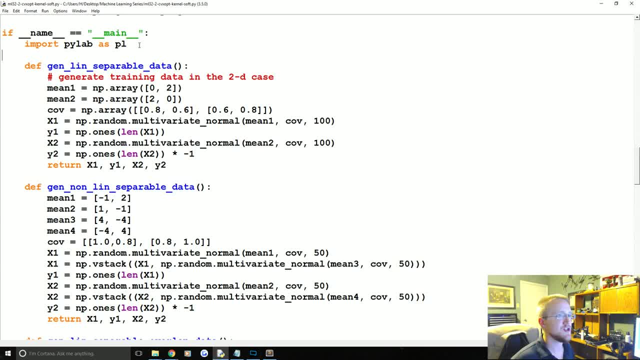 Bringing in PyLab here, really showing it's age, but anyway, brings that in. I think this is from like twenty ten. anyway Brings in PyLab, okay, and then generates linearly separable data. so this will be data that you can do, no kernel and it can be a hard margin classifier. 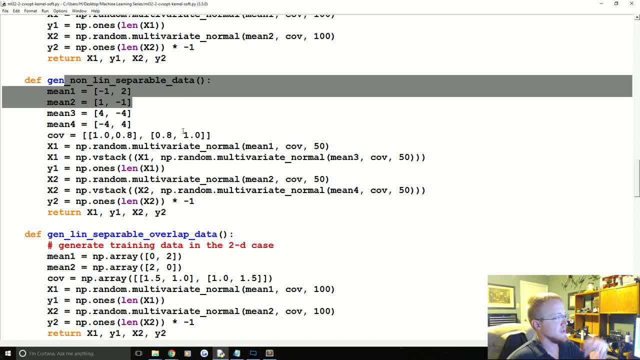 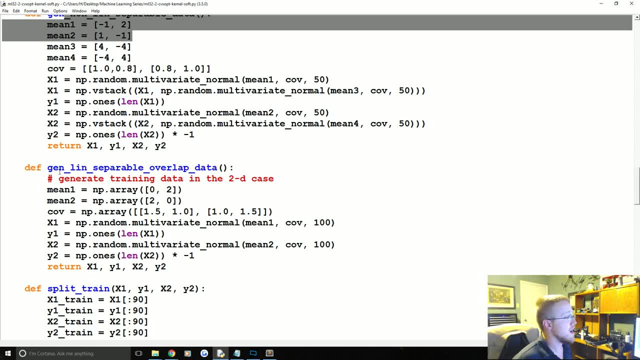 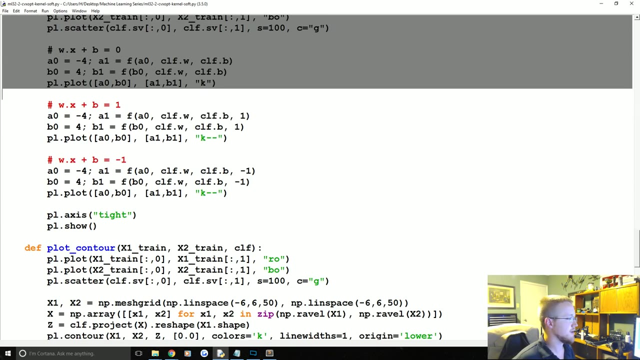 this one's non-linearly separable data, so this would be data that needs a kernel. right then we've got generating linearly separable but overlapping data. this is data that needs a soft margin. okay, this splits up training data, this makes testing data, and then this is just some nice code that will plot a. 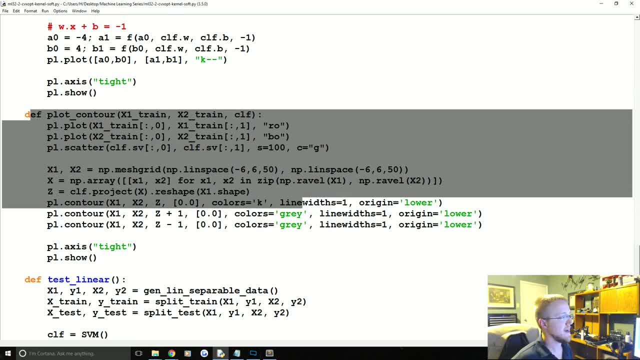 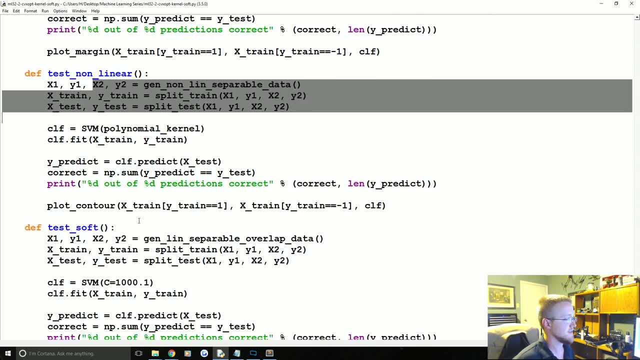 linearly separable data. this one is for anything that's going to have a kernel, that's going to be all kind of contoured around, and then here's some functions to actually test all of that stuff. i've just went ahead and put them down here, so let's just run through it really quick. so testing. 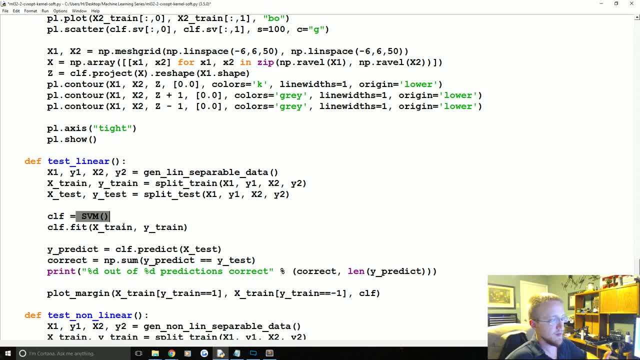 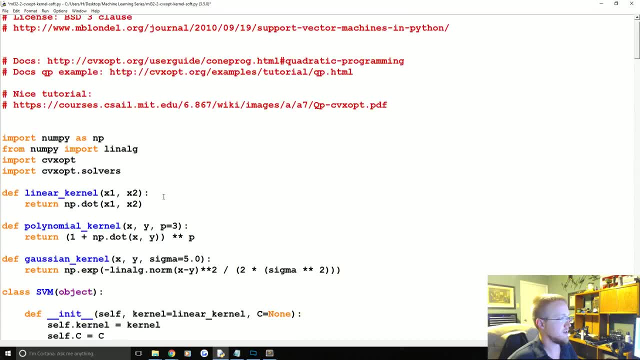 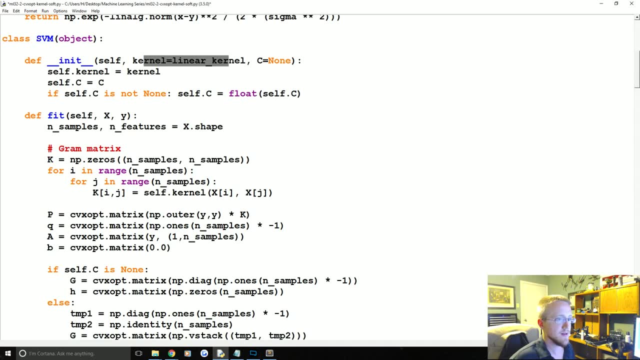 linear. all he's going to do, basically, is just there's no penalty parameter, right, so it's hard margin, uh, and the default kernel was a linear kernel- come on mouse wheel, right? so if you wanted to change that, you could change that if you wanted. uh, but it's just defaults to linear kernel, so we can go. 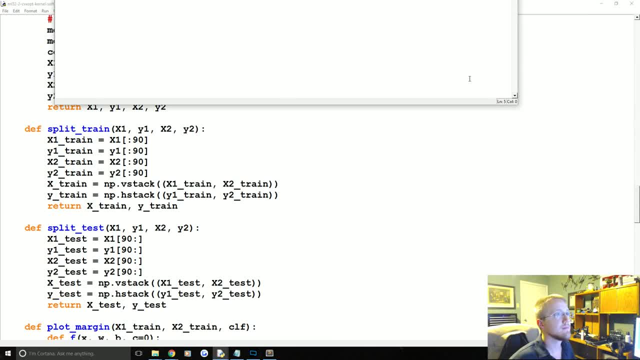 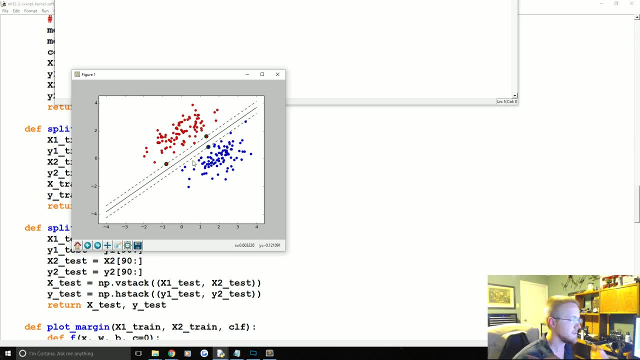 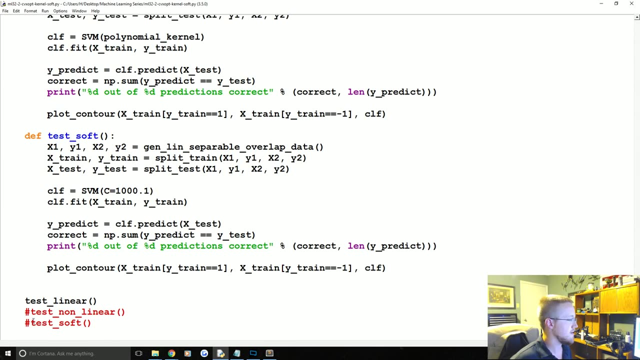 ahead and run that really quickly. sure enough, there you have it. you've got your support vectors here. a nice low number of support vectors. we're pretty content cool, successful. it's a simple, simply separable data set as well, anyway. and then coming on down the non-linear: i think by default non-linear was using the gaussian kernel. i just changed it to. 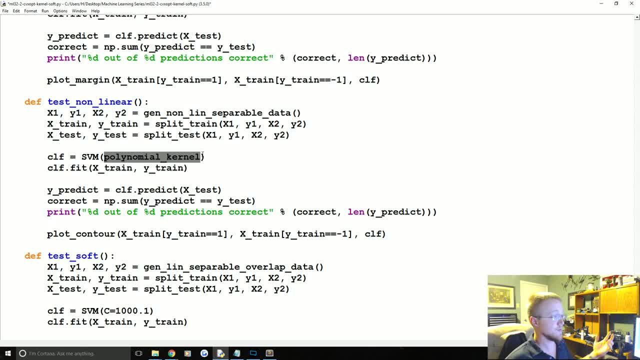 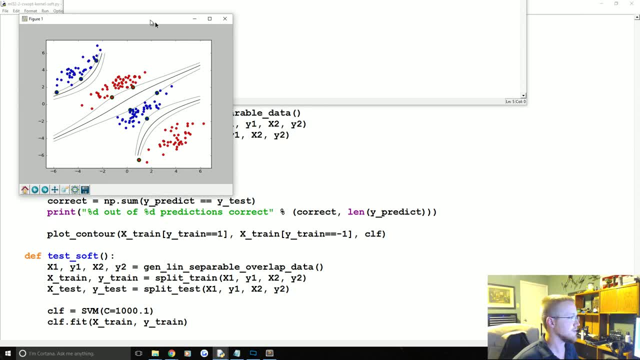 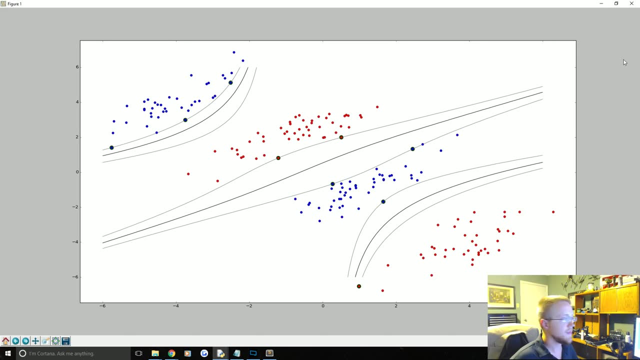 polynomial, since we didn't actually talk about the gaussian kernel. doesn't really matter, but just note i did make that change. so we're just using a polynomial kernel rather than the original. but, as you can see, you still get corrected or correct separation of that data. and one thing, um, i guess i'll show it really quickly if you want like a visualization of 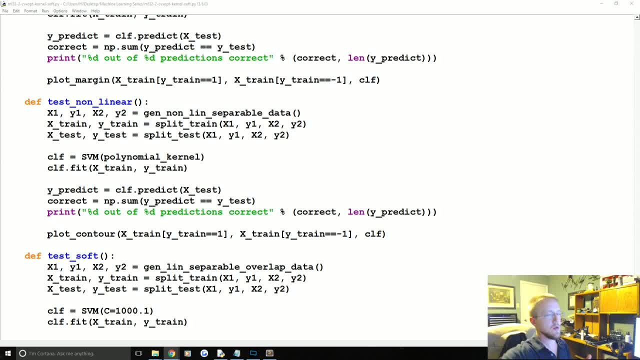 like how that were like how do you translate to another dimension and then pull it back down to two dimensions, like so, how do you go from three dimensions, let's say, down to two dimensions and get those contours? a good thing to google is svm kernel visualization. i'll go ahead and pull it up. 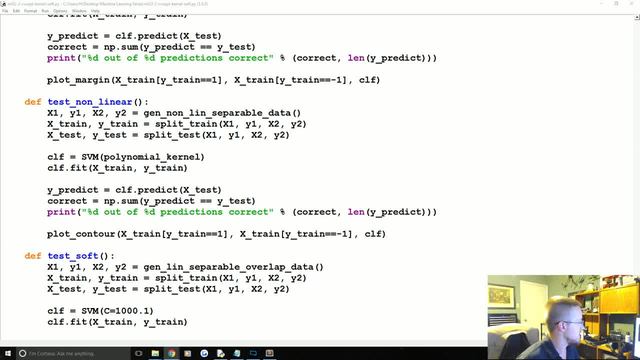 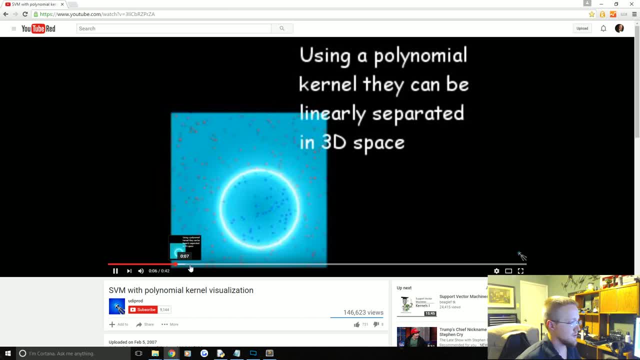 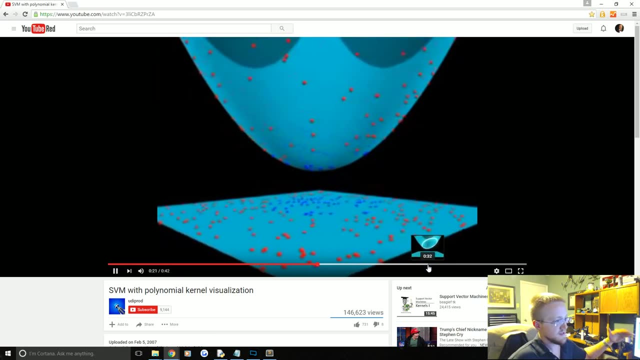 but you can look at it yourself too. let me pull up and change the speed to pull this on over and i will play that. so that's your 2d data set and then he's about to transform it- there it is- into three dimensions and then it's linearly separable. so we 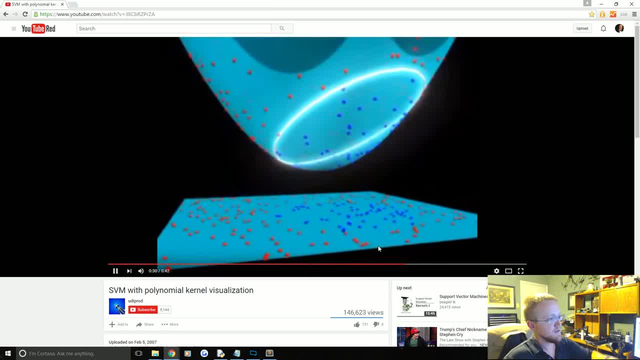 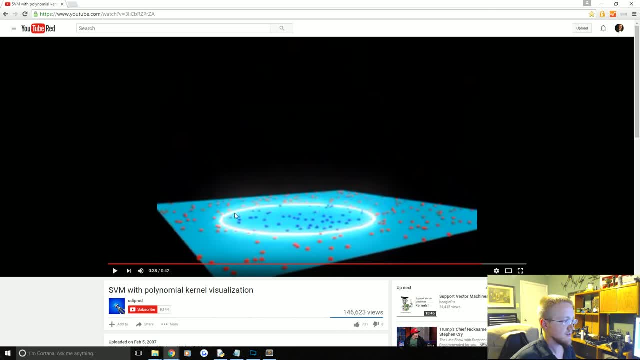 slide in that hyperplane, great. and then you can see you've added that just basically the circle that it passed through, and then you can see, like, basically at the end of the day, back in two dimensions. it's just a simple circle for the separation, so it's kind of a useful visualization. 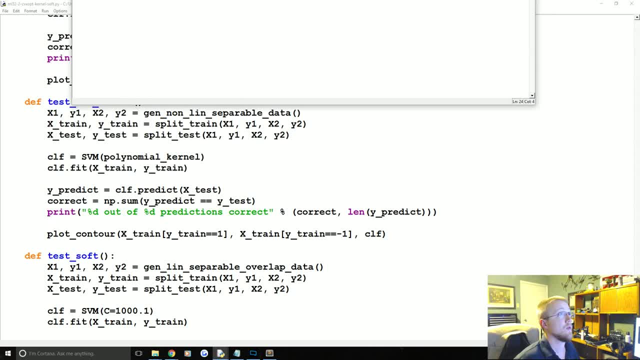 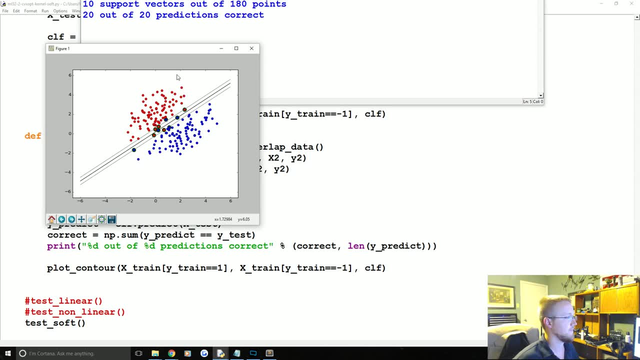 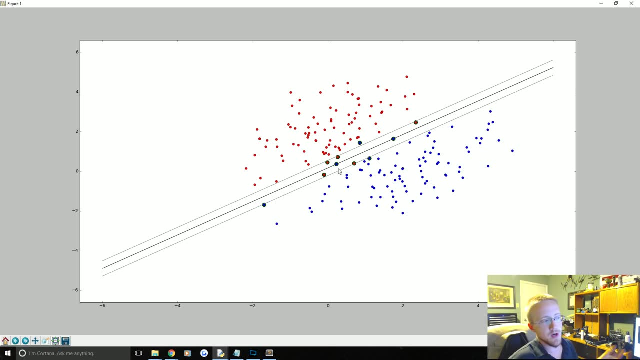 for for how that process actually works, and then finally, we'll do go ahead and do the soft margin run that real quick, okay, so, as you can see, um, it is, you know, totally linearly separable data. it's just that there's a little bit of overlapping going on there. not a huge problem. 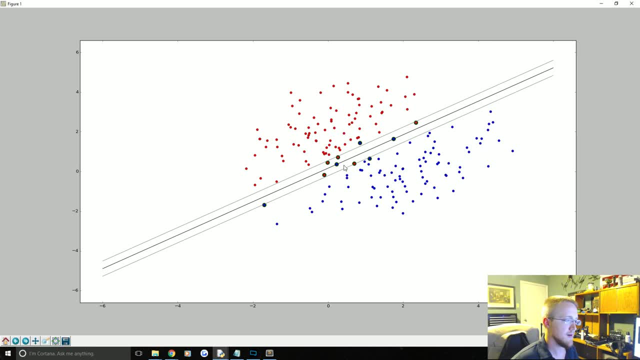 still don't have too many support vectors, so we're doing fine, without it being soft margin. this is just simply not linearly separable, but you could. you could have a kernel that solved that problem, most likely. so anyways, um, that's all the examples again. you can kind of poke on through and just see. 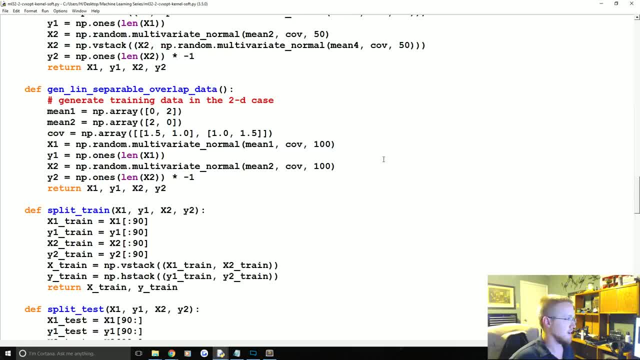 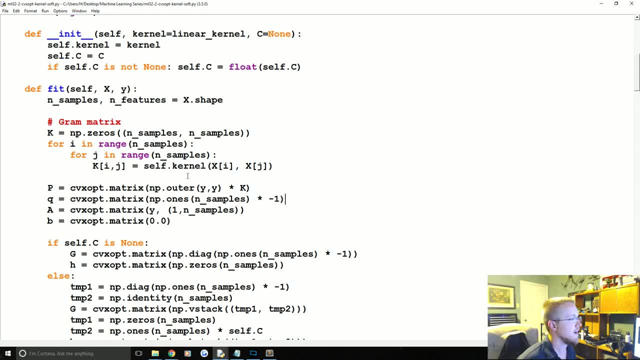 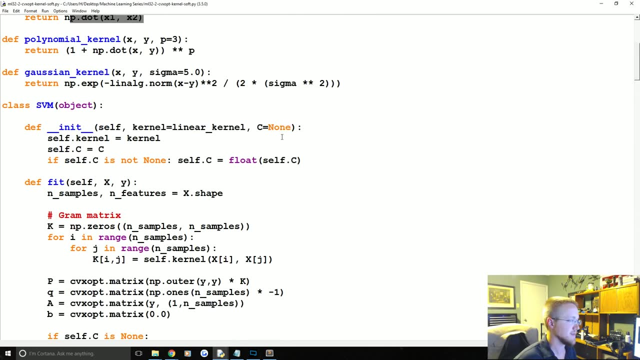 how the kernels are affecting it, and in fact you could even um come up to. well, we can do, yeah, okay. so right, right here you can see, selfkernel is always going to be used. it's just the case that if it's a linear kernel, it's just the dot product of the, the two. 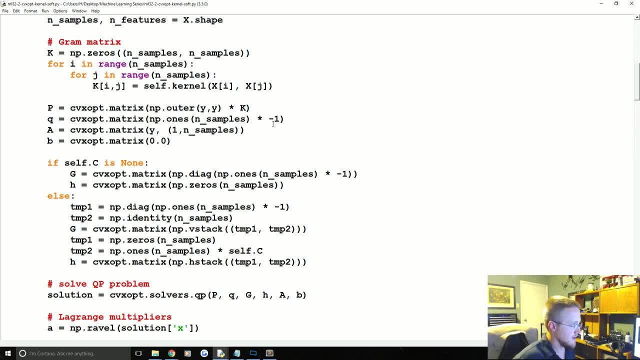 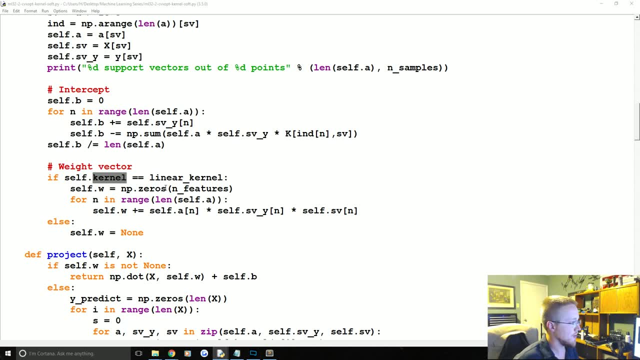 values. um, then you've got. i believe there should be probably one more kernel in the prediction, most likely, oh well, the weight vector. okay, yeah, if it's a linear kernel, then it's just two rows, but if it's not, um self, w is just none in that case. and then 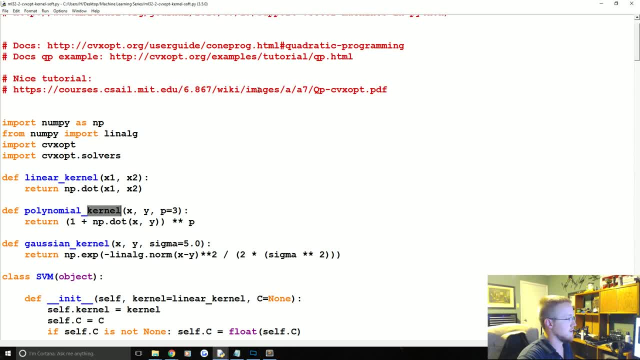 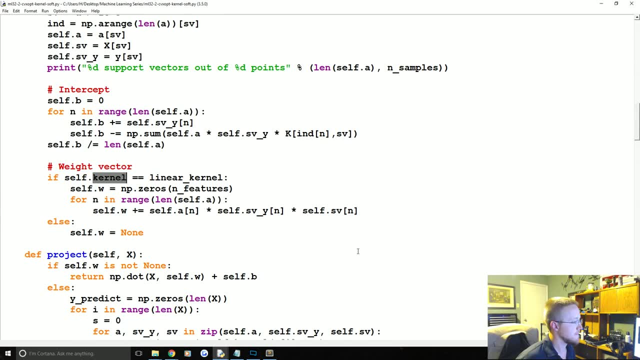 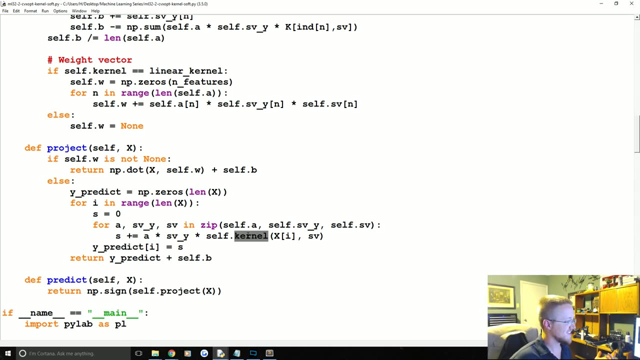 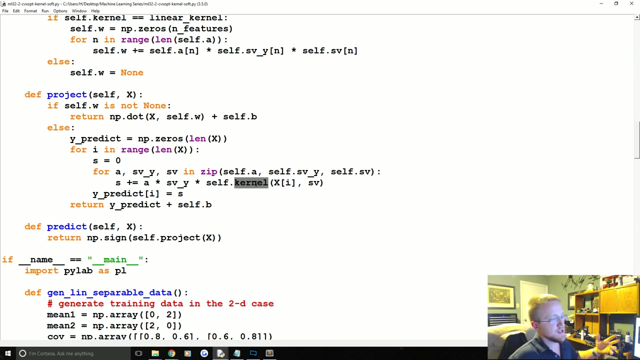 oh, that's it, let's see, just making sure we actually cut, okay. so anyways, um, i knew there was enough. i was actually in the projection, know why i wasn't finding that, but anyway i had to go down there myself. so, yeah, obviously in the projection you'd also have to take your that feature set. you're trying to predict and translate. 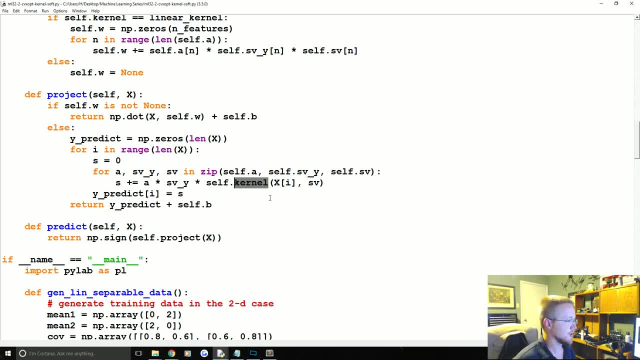 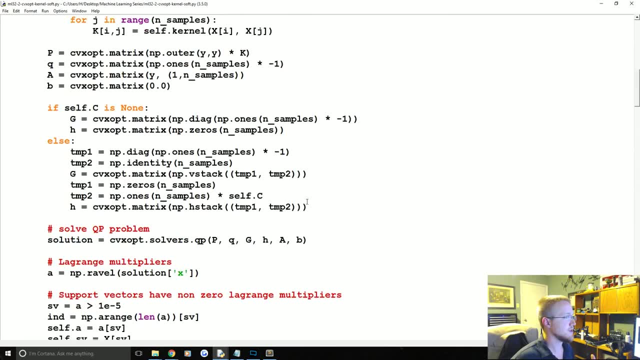 that as well, grab that kernel. but anyway our kernel value i suppose. so that's just like a quick one through the code. if you have questions or whatever, feel free to leave them below on this code in the next tutorial we'll kind of wrap. we will for sure wrap up the support vector machine. 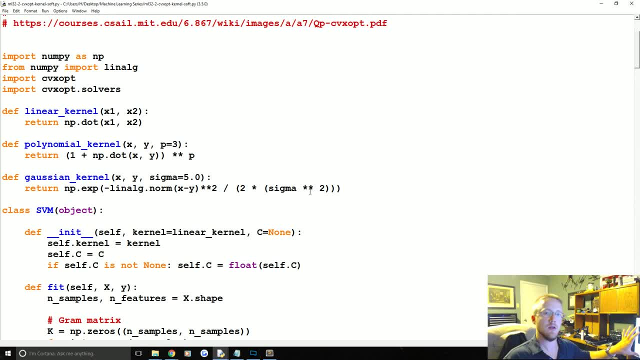 we're going to go through all the parameters from, for scikit-learn's support vector classifier, because, one, it's a decent review, but two, it actually will help us cover a few more concepts that we actually haven't covered and kind of bring you up to speed as far as what people are doing. 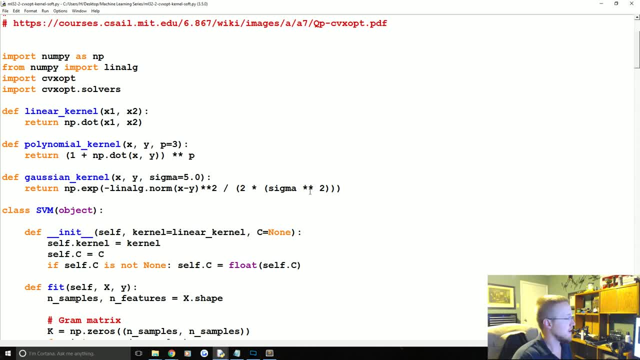 nowadays for solving the svm, so that's pretty useful. also, we'll talk really briefly right at the beginning about you know what do you do when you know support vector machine is supposed to be a biomechanical machine and you're not going to be able to do that. so we're going to talk about 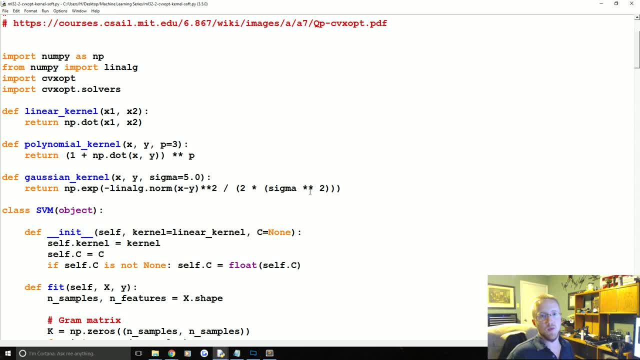 binary classifier. so can you? actually, how do you classify more than two classifications, like, let's say, you've got three classes? how do you actually do that? so we'll talk about that and then we'll launch into the svm parameters and all that. so, anyways, if you have questions, comments.